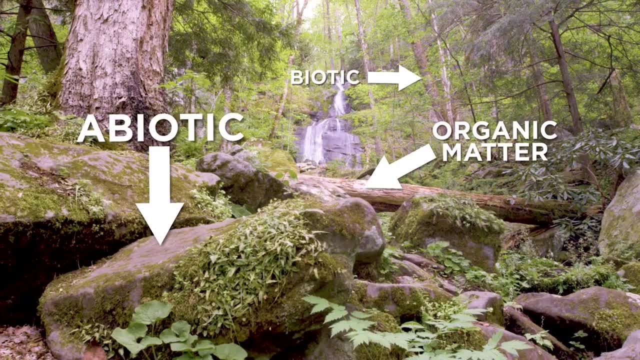 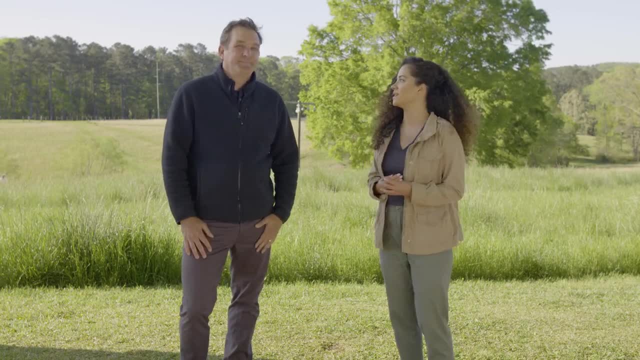 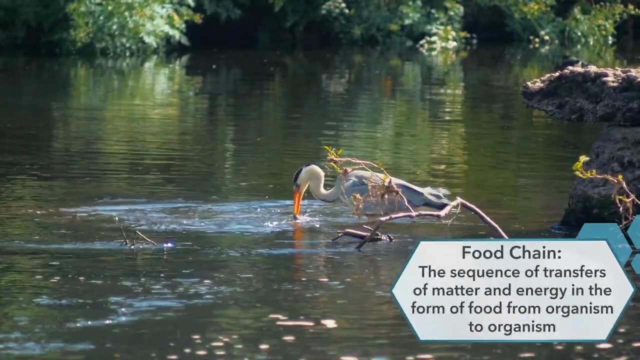 and the non-living things are the abiotic component, and they all, in one way or another, depend on each other. So how does energy flow through the system? Energy flows through an ecosystem via the food chain. The food chain, Yes, the food chain. It's the order in which organisms eat other organisms. 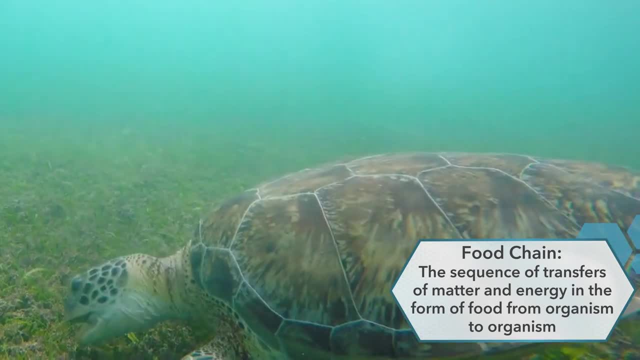 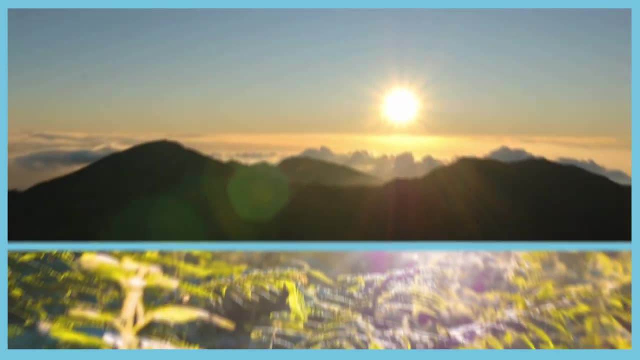 in the environment, and that's where nutrients and energy is transferred from one organism to another. So the cycling of energy begins with the sun, which enables producer organisms, such as plants, to make their own food. It then goes through consumers and ends with decomposer organisms. 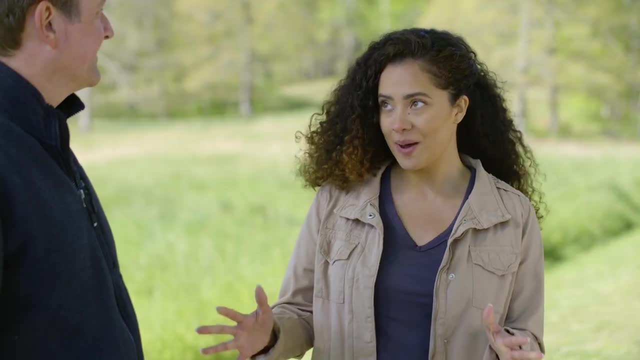 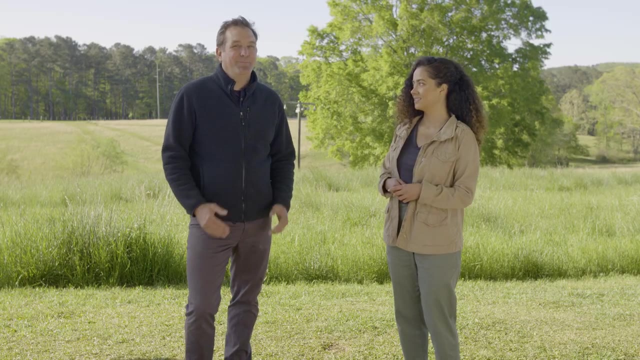 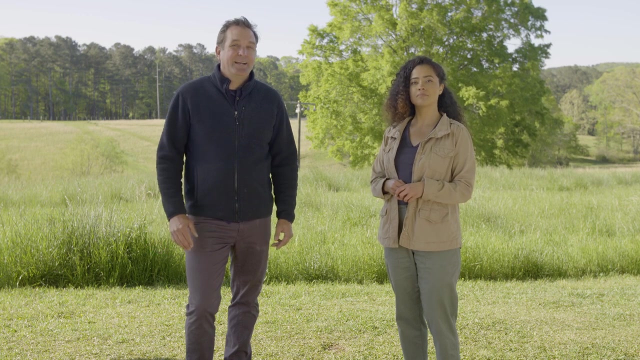 that feed on the organic matter and so on. What about matter instead of energy? Does that flow through an ecosystem too? No, actually matter cycles from one state and place to another before returning to its original state. But a cycle is not like a big, continuously circling hula hoop. There are lots of pathways. 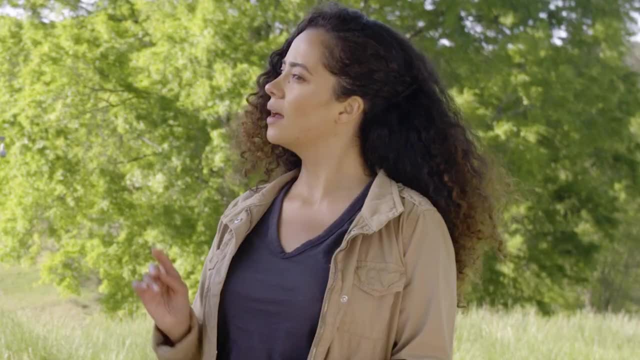 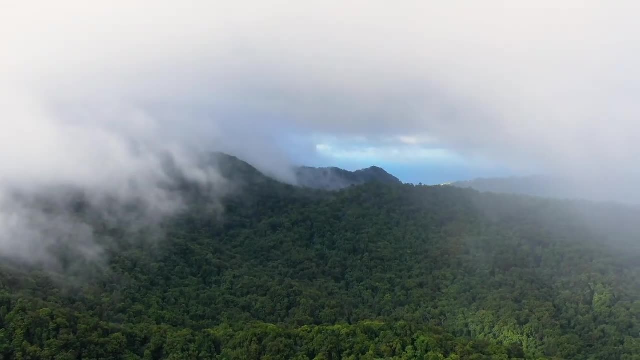 lots of directions to go and lots of places to get stuck along the way. What do you mean by that? Well, for instance, a fish might drink water and later pee it out again. then the water in that drop of pee might get evaporated into the atmosphere and spend a while. 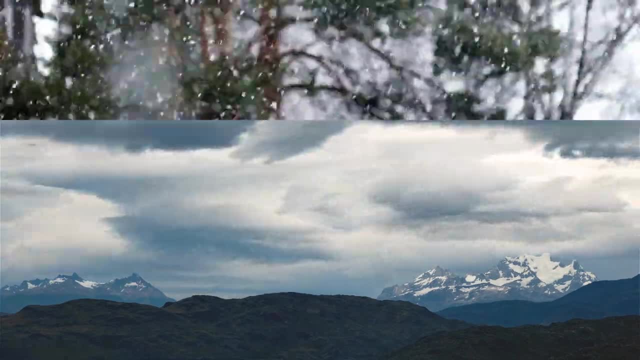 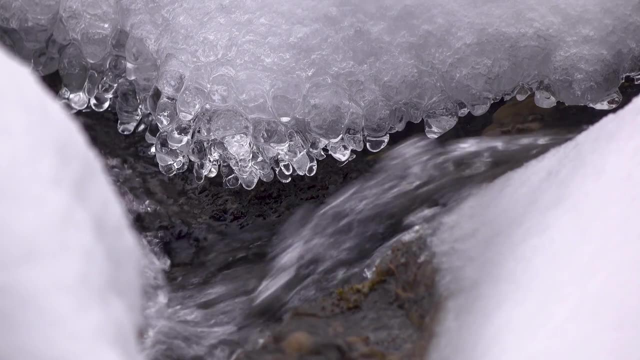 getting stuck in a cloud that gets blown around by the wind to a cooler place. Later, that drop of water might fall back to earth as a snowflake that gets piled on by other snowflakes until pressure turns it into ice. It could be stuck as ice for a long time before it ever has a chance to melt, and 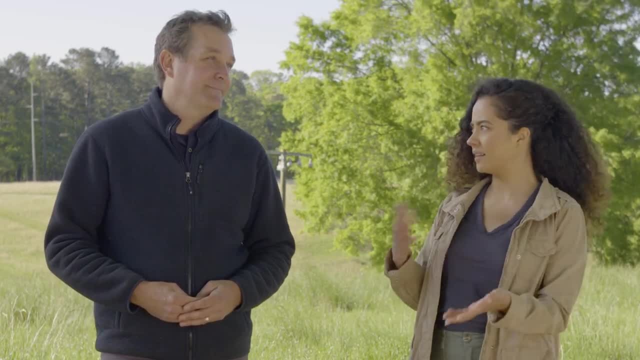 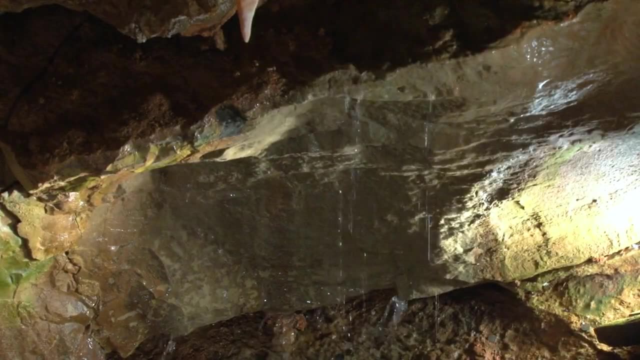 flow into a stream, And if it falls into the ocean instead, I guess it would have to cycle again before it has a chance to land back in the stream. right, Right. all the water that gets stuck for a while in oceans, underground in ice or in clouds during the water cycle would then start from there. 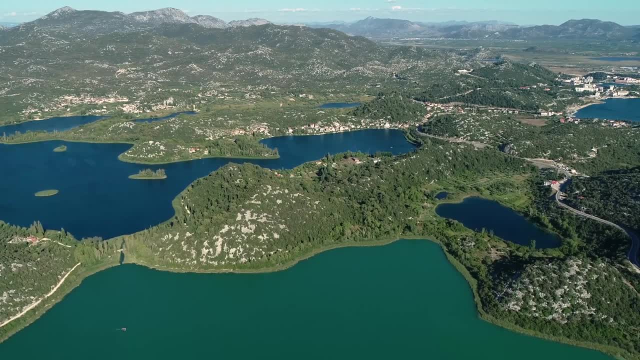 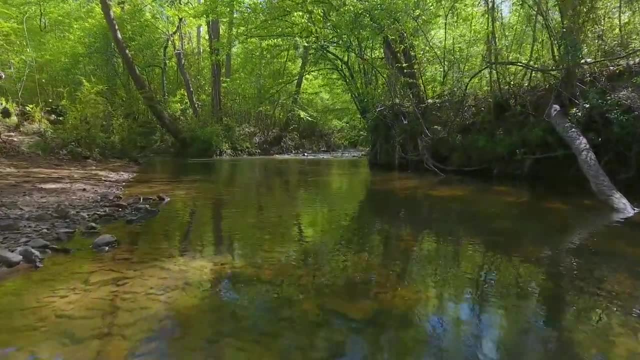 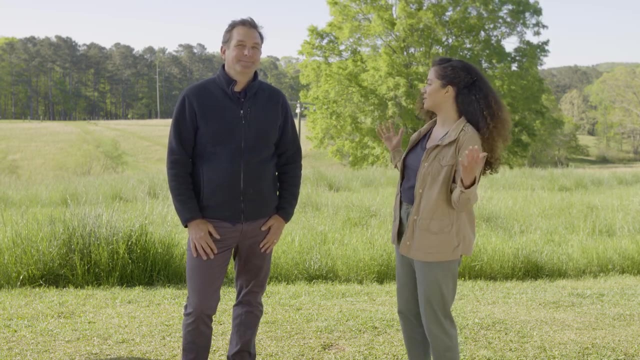 only about three percent of it is freshwater in the world, and about less than one percent of that fresh water is available to us as humans in the form of streams, rivers, lakes, at any given time. wow, well, i'm quite excited to dive into some fresh water today. where we are now is so 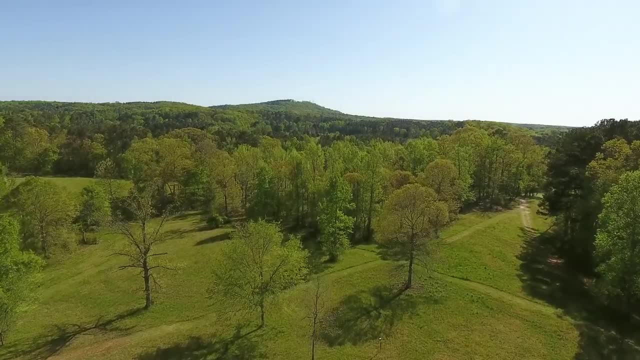 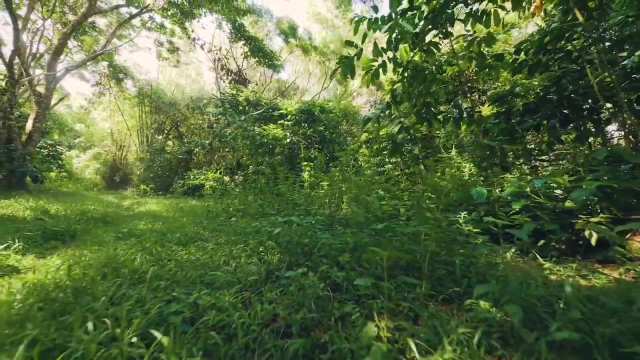 so beautiful and it seems like the perfect place for what we're investigating. uh, definitely it's. it fits the bill for a few reasons. some ecosystems are terrestrial, meaning they are land-based, and some ecosystems are aquatic, meaning they include a body of water and, like everything else, these 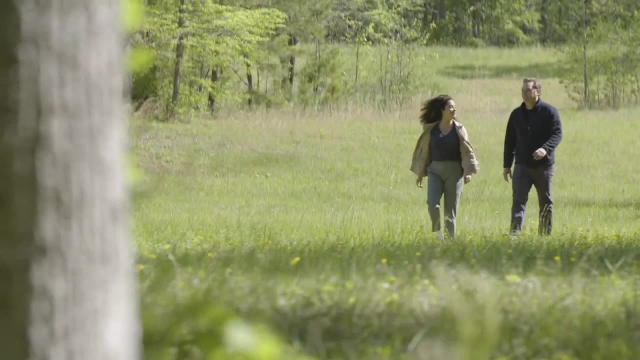 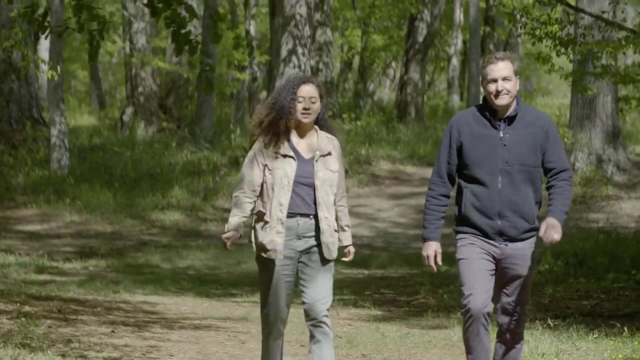 ecosystems impact one another, so where we are located now, which is a park in cobb county, it includes streams that are part of a larger watershed in the area. it's a great place to explore a functioning ecosystem and i imagine that it is a good thing that i didn't see any 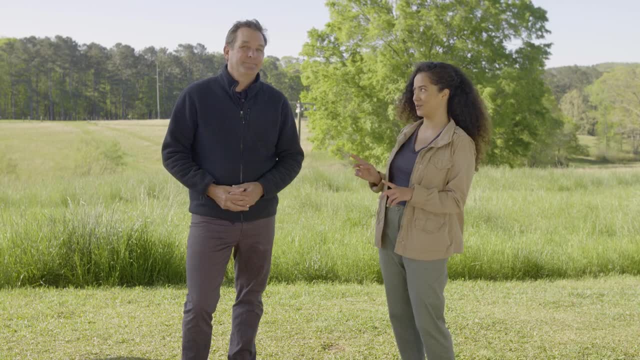 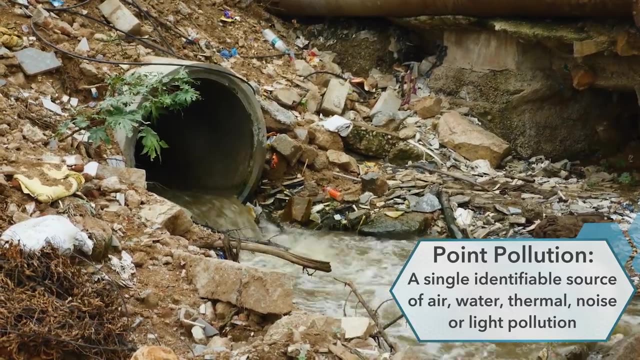 factories around here. so that probably means there's no pollution, right? well, water pollution doesn't only flow out of pipes, called point source pollution because you can track it back to that point. but non-point source pollution is when rain flows across the land and into ditches and then 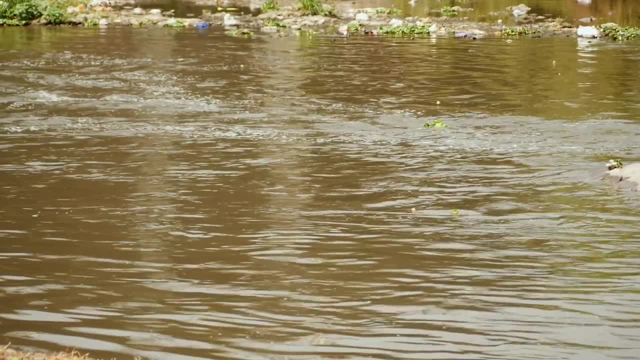 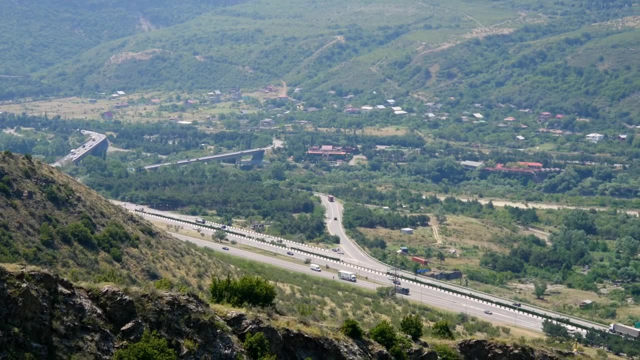 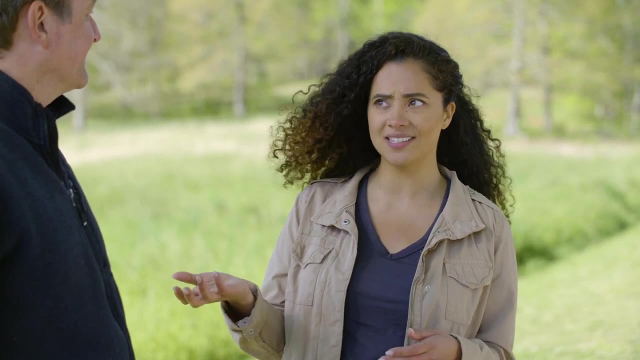 into creeks and rivers. it dissolves and carries all sorts of pollutants with it. do you mean things like litter? yes, but also fertilizer, animal poop, oil that is leaked on roadways, and so forth. animal poop do you mean like from wildlife farms, ranches feed lots? yes, but from pets too. 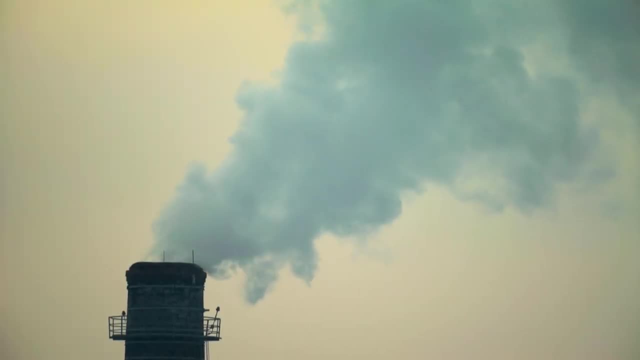 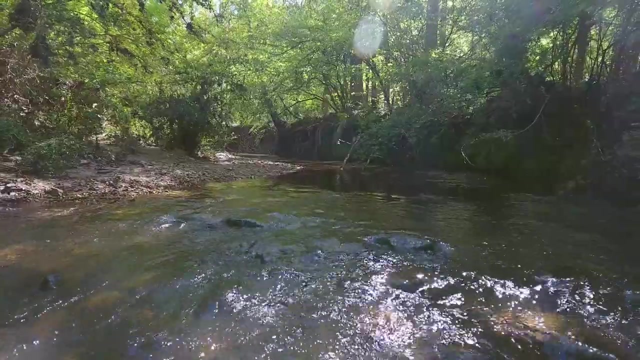 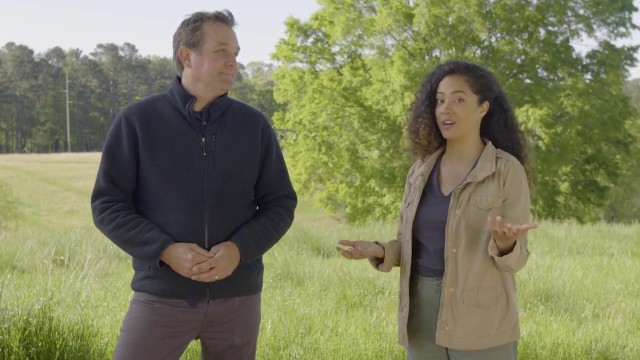 everything from erosion, mining and even air pollution gets into the water eventually, through runoff. everything that pours out of pipes, falls on the ground or gets dumped into drains eventually washes downstream into creeks and rivers whenever it rains. wow, well, as a georgian, i'm very interested in whether our rivers and streams are healthy aquatic ecosystems. 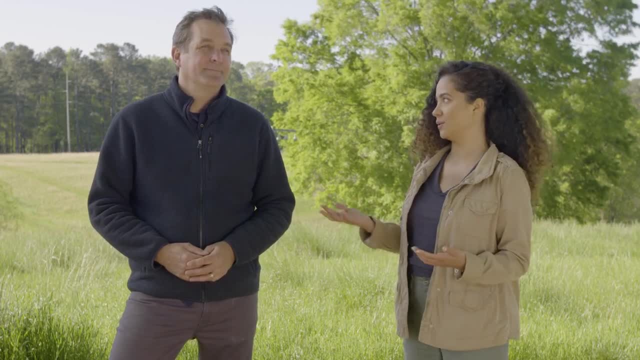 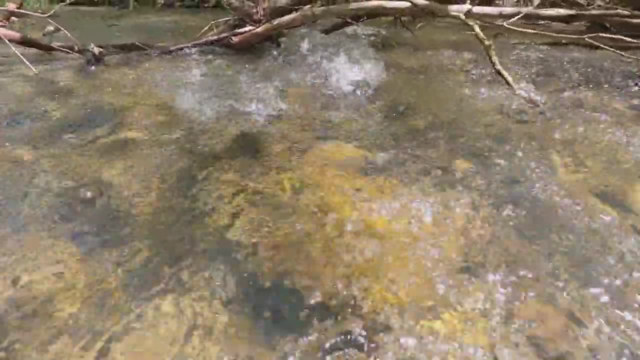 so how can we determine whether a body of water is polluted? well, there are four main ways that students and other volunteer groups can assess the health of water. there's visual surveys, which students can learn to read a river or stream by its color, frothiness, clarity of water and 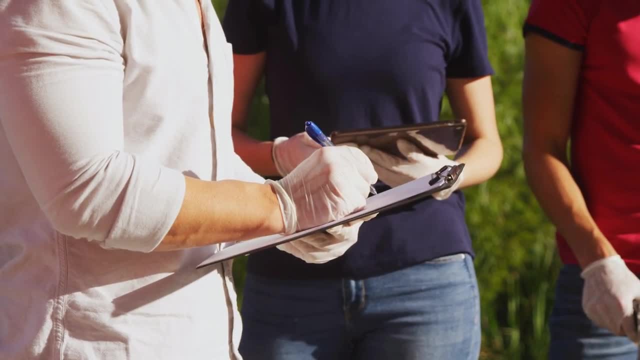 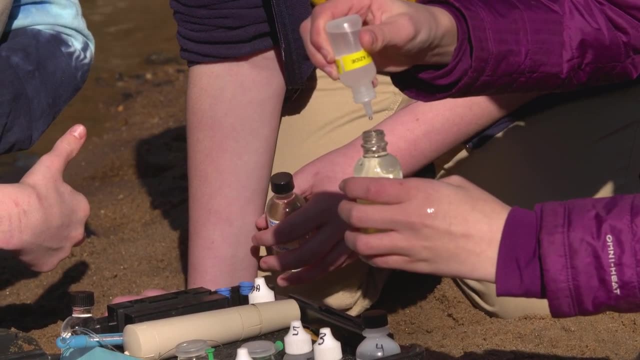 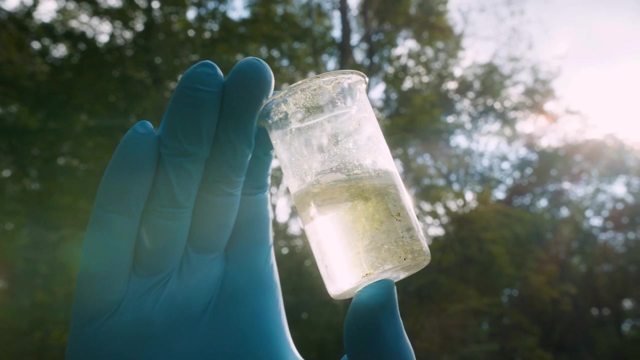 clarity and smell and they can report spells and contaminants that they might notice, and there are physical and chemical tests which students can also do. the main things we test for are dissolved oxygen content of water, because fish and other aquatic organisms need to breathe underwater. we also test for phosphorus and nitrogen, because they act like fertilizers and can cause overgrowth. 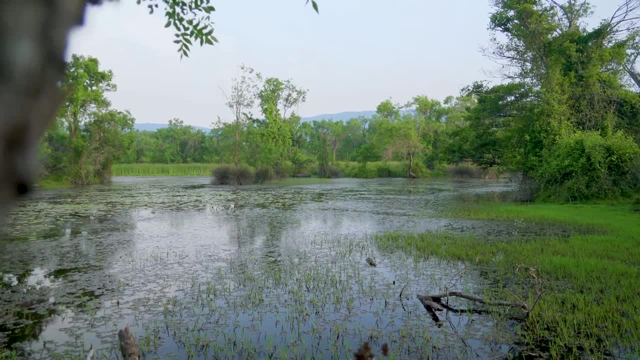 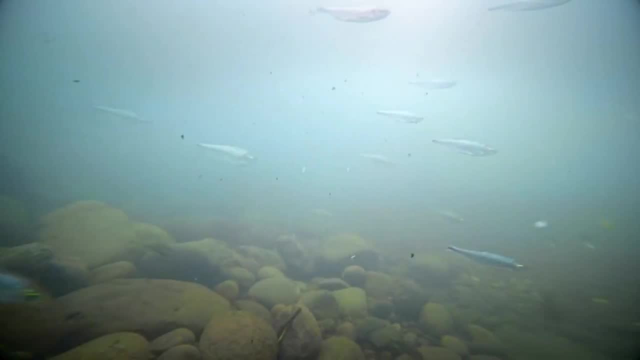 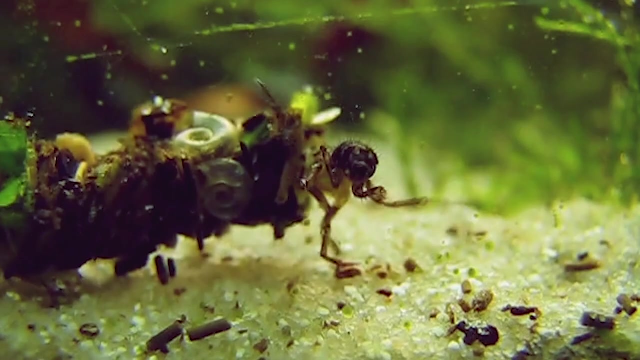 of aquatic plants and algae. now, all that plant growth requires oxygen from the water, and then when the plants die, it robs even more oxygen from the water, so fish and other organisms can suffocate. there's also sampling of water to look for little aquatic organisms that are bio indicators of water quality, and that's because they're either.